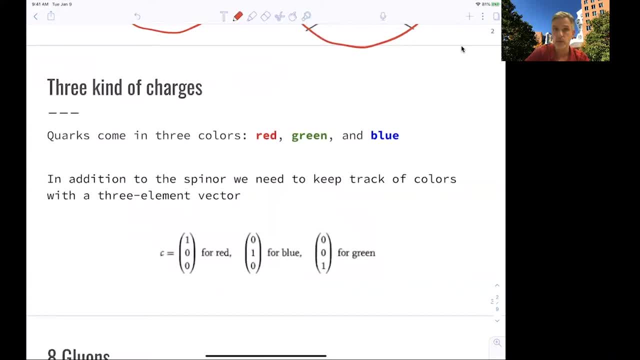 Meaning that the quarks come in red, green or blue. So we have to keep track of this when we write down our amplitudes, our matrix element. So we do this by just introducing a new vector. I call this C here. Very simple, A three-element vector for those three colors. All right, 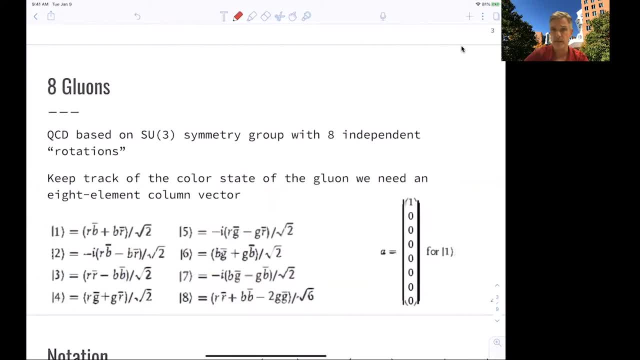 But how about the cloon itself? So QCD is based on a symmetry group which is called SU, So it's basically a rotation in a three-dimensional space. There's eight independent rotations, such rotations, And what you want to think about is just moving quarks from one color. 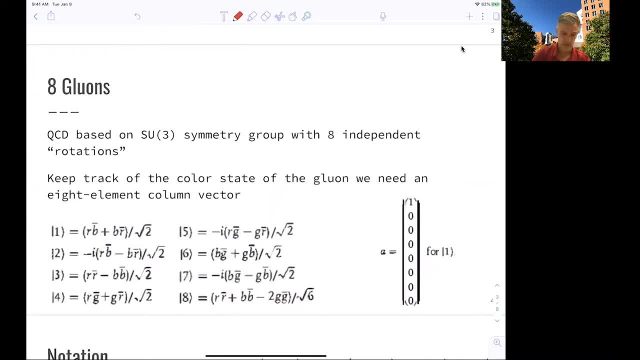 state into the next So you can write them down as I show here, And we do this in linear combination of color and anti-color. All right, If you want to keep track of this, we do this in this form. We have a vector which is eight elements And the gluon is one of those components. This is 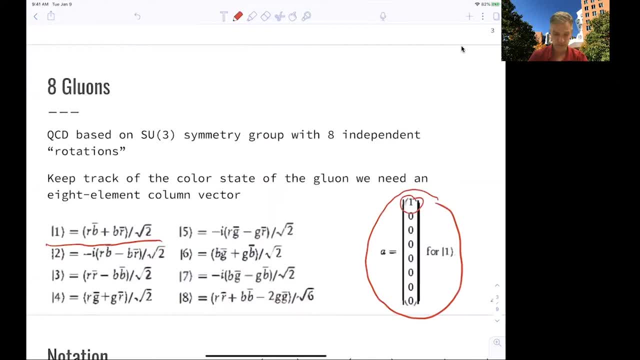 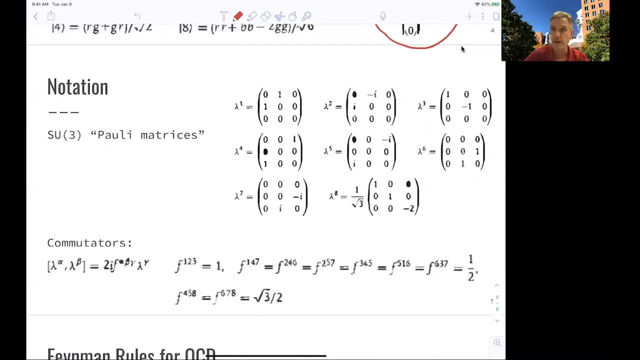 given here for this very first one. OK, So let me introduce the notation here. Literally we were introducing Pauli matrices, but not for SU as a symmetry group. for SU They're called the Gell-Mann matrices And they're just written here Again. those are the rotations I was just talking about. 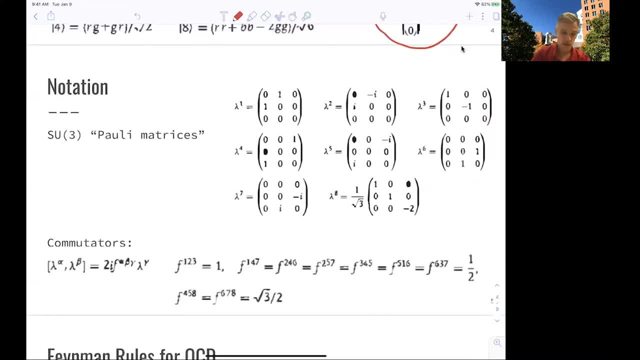 Those are the rotation from one color state into the next. There's commutator relations for this. So if you have two of those Gell-Mann matrices and you try to write down the commutator, you find this is two times R. 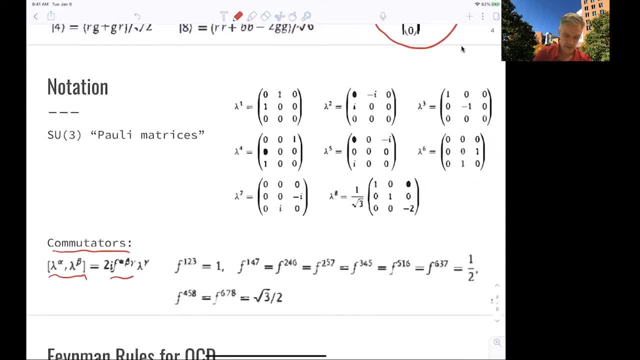 I times this structure constant times the next Gell-Mann matrix. So if you're just thinking about how many combinations are there, there's eight matrices. We have eight times eight times eight combinations of those constants here, And so it means that there is 512 of those constants. Most of them are zero. 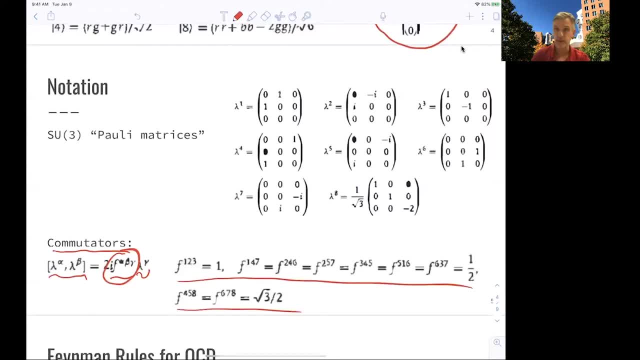 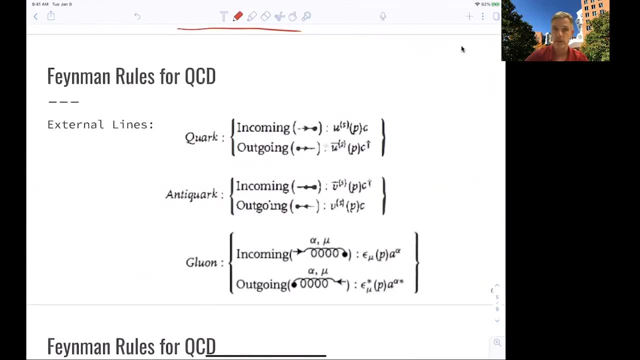 And the ones which are not zero. they're listed here, So we have two combinations of those. All right, So now we are ready to just write down the QCD Feynman rules. Again, we start from the external lines. So for the incoming quark or outgoing quark, 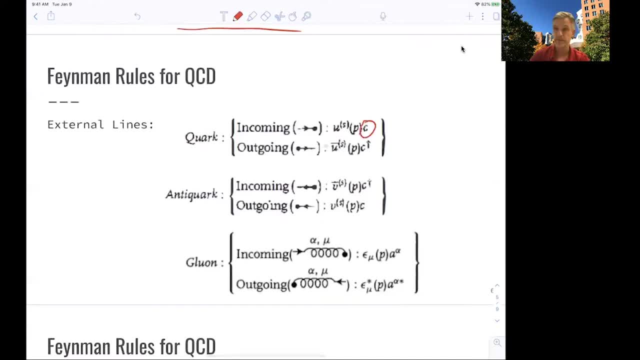 we write our spinor And then we keep track of color. OK, We do this for quarks And we do this for anti-quarks. in the very same way For the gluon. now we have to keep our polarization, keep track of the polarization of the gluon.